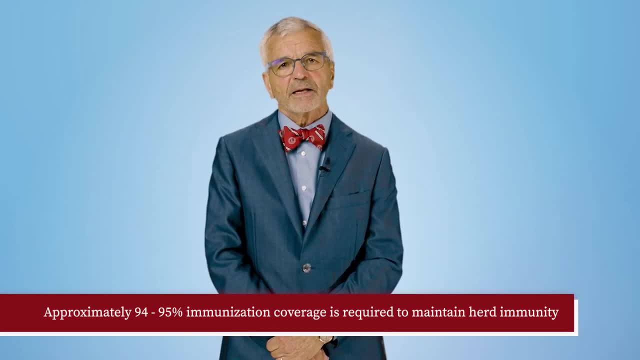 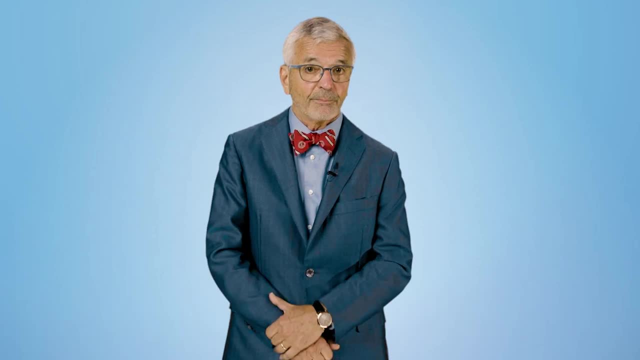 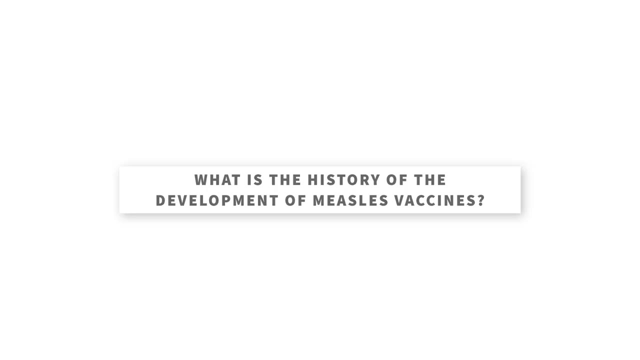 Approximately 94 to 95 percent immunization coverage is required to maintain herd immunity, meaning broad population immunity, and to interrupt continued transmission of measles. What is the history of development of measles vaccines? The first measles vaccine was the first to be developed in the United States. The second measles vaccine, which was created by inactivating- that is, killing the virus, was developed and licensed in the United States in 1963.. The current vaccine is live attenuated, meaning a weakened vaccine. So it's live virus, but the virus has been weakened in the laboratory. This was introduced in 1968.. The measles vaccines used in the United States now are combined with mumps and rubella and the vaccine is called MMR- measles, mumps and rubella, or combined with mumps, rubella and varicella. Varicella is chickenpox And that's the MMRV. 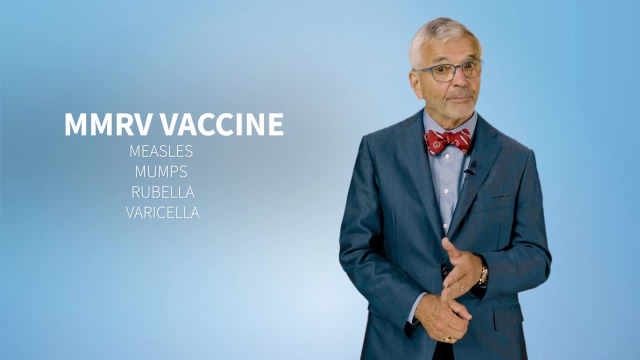 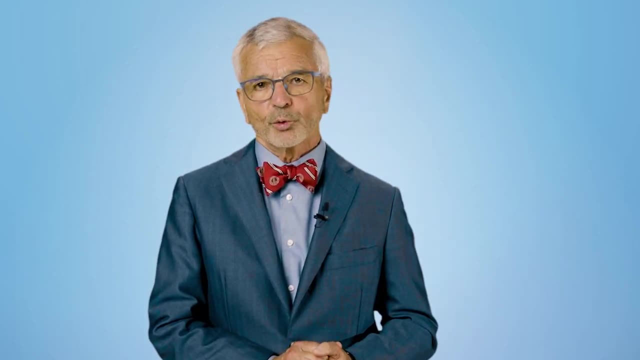 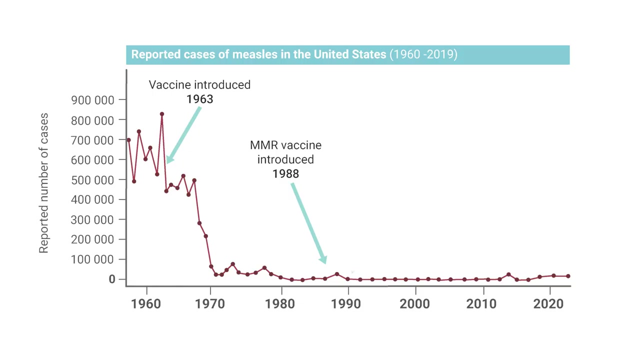 vaccine: measles, mumps, rubella and varicella. For many years, only a single dose of measles vaccine was given to young children, But because of occasional infections still occurring, a two-dose strategy was adopted in the United States in 1989.. And now the standard vaccination. 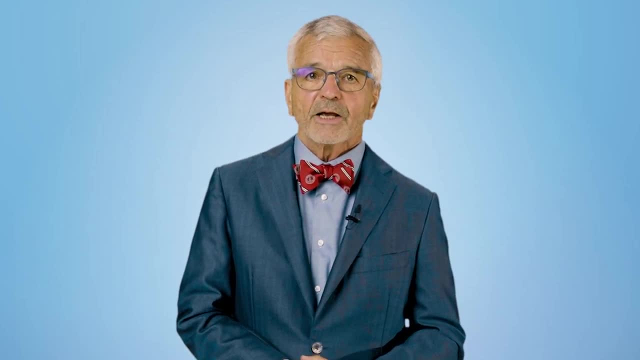 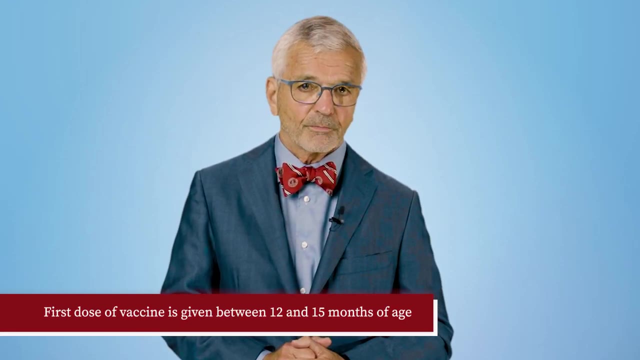 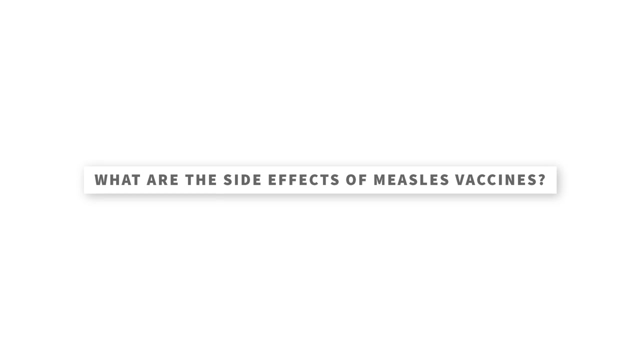 schedule for measles prevention and control is the administration of two doses. The first dose of vaccine is given between 12 and 15 months of age, and the second dose is given between four and six years of age. What are the side effects of measles vaccines? Well, as is true of all, 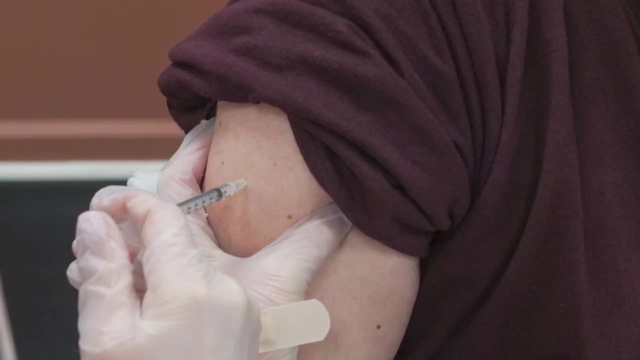 vaccines, there are some side effects. One of them is that the measles vaccine is not relatively safe for people with symptoms that are injected into the body. There may be some local discomfort from the needle. So a little bit of pain, sometimes a little bit of swelling. 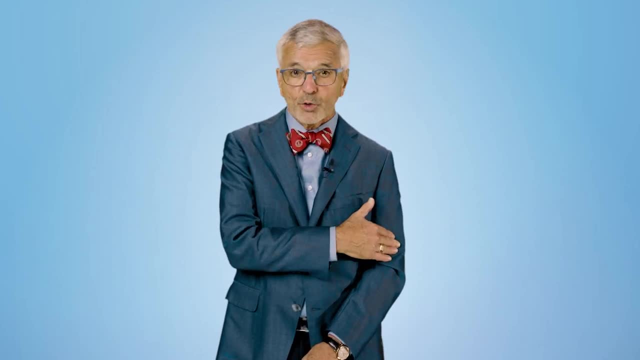 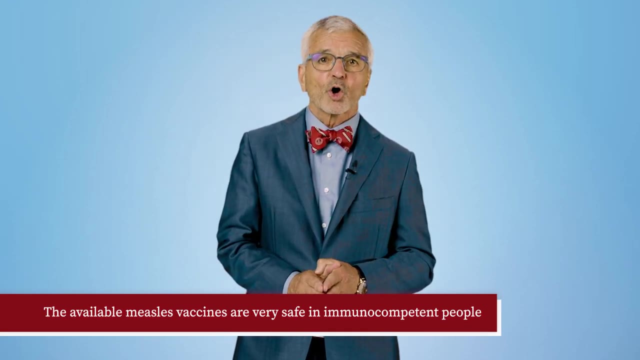 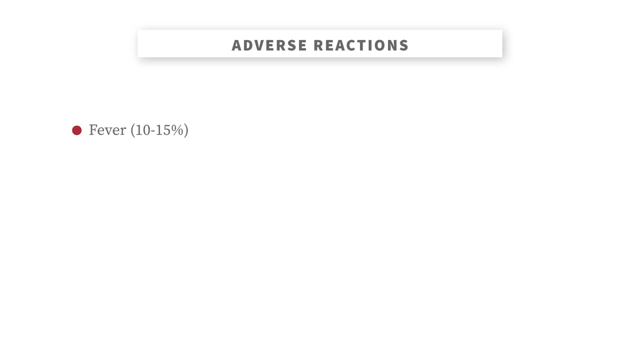 or redness that lasts typically a day or two days. The available measles vaccine are very safe in immunocompetent people, people with a normal immune system. The adverse reactions to the vaccines may include fever. usually about 10 to 15 percent of recipients There may be a transient, that is, a temporary rash. 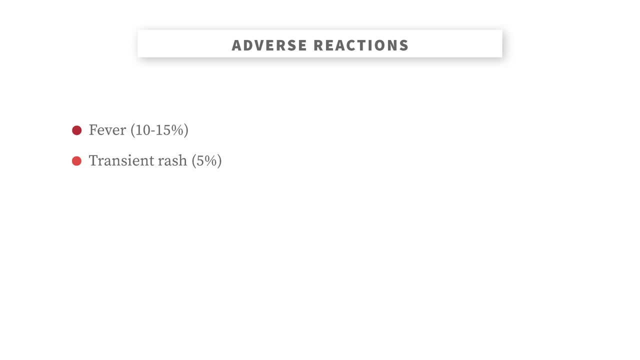 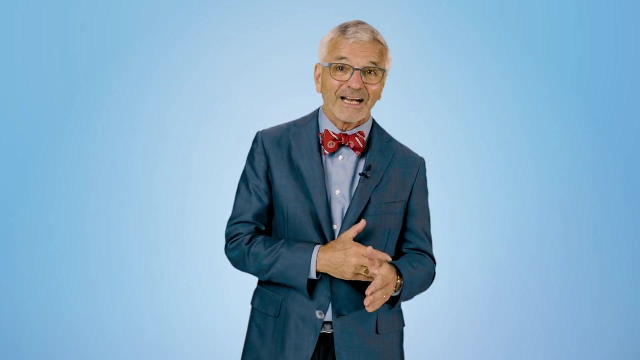 that occurs in about five percent of vaccine recipients, And these symptoms- the fever and the rash- usually occur about a week to two after the vaccination has been given and they persist for one or two days. The reason they occur one to two weeks after the vaccination is remember. 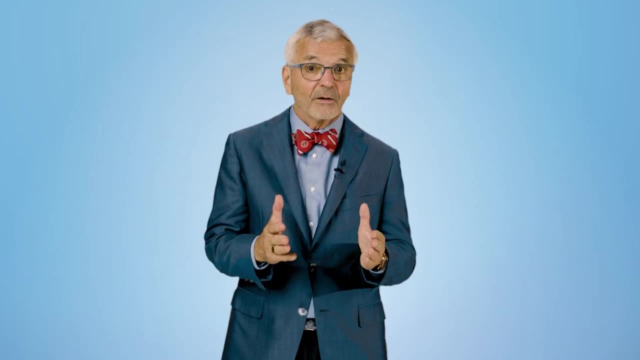 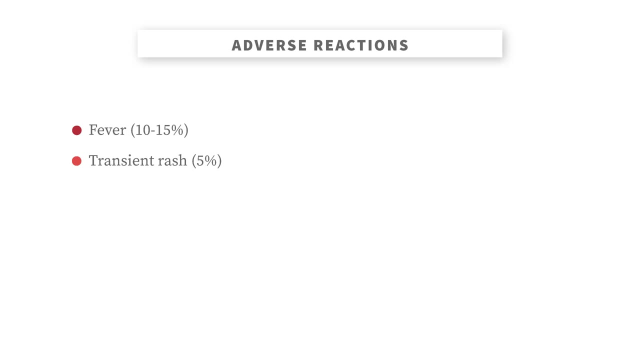 the vaccine is a live but weakened form of the virus, So the vaccination may imitate, but at a very reduced level, some of the symptoms associated with measles itself. Brain inflammation or encephalitis after a measles vaccine is very rare. It is estimated to occur. 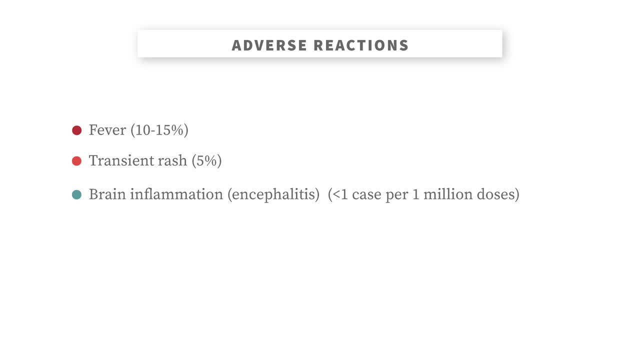 less than one time in one million recipients of a measles vaccine. Other serious adverse events also are unusual. These include febrile seizures, that is, seizures occurring when the child's temperature rises. This is estimated to occur about one time in every 3,000 recipients of the vaccine. 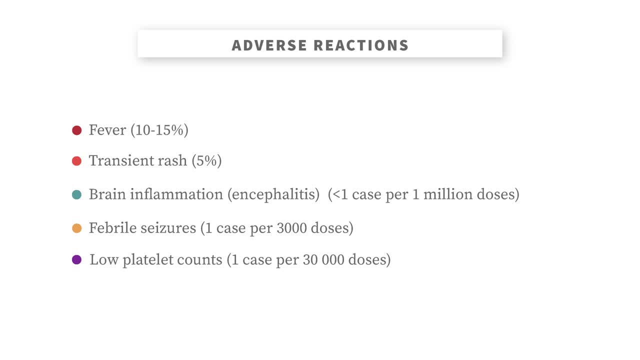 Low platelet count may occur. This is estimated to be at about one case per 30,000 doses of measles vaccination And rarely anaphylaxis, which is that which you can get after a bee sting, you know, with a rash, some swelling. 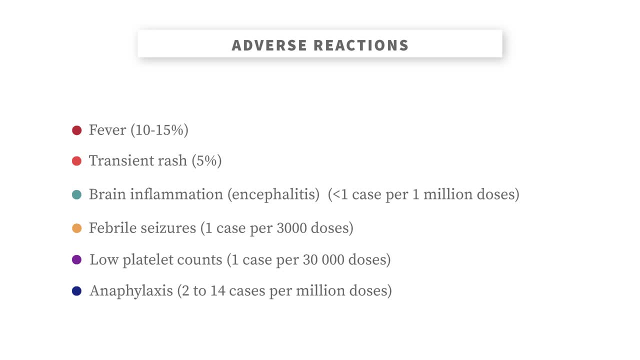 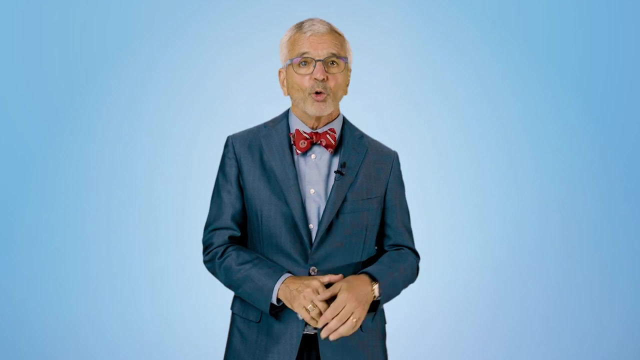 Maybe some difficulty breathing. It's called an anaphylactic reaction. That occurs somewhere between two and 14 times for every million doses of vaccine, given Allergic reactions related to allergies to egg or egg products or to the neomycin, a small amount of which is in the vaccine. 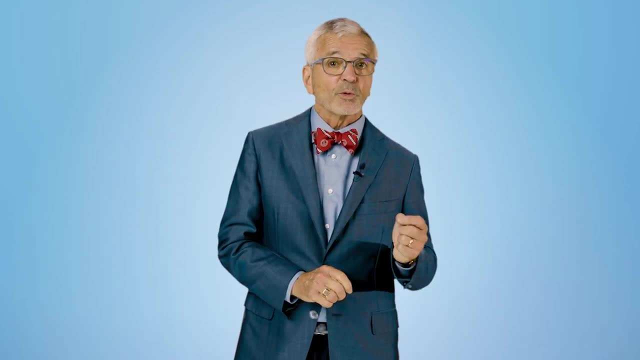 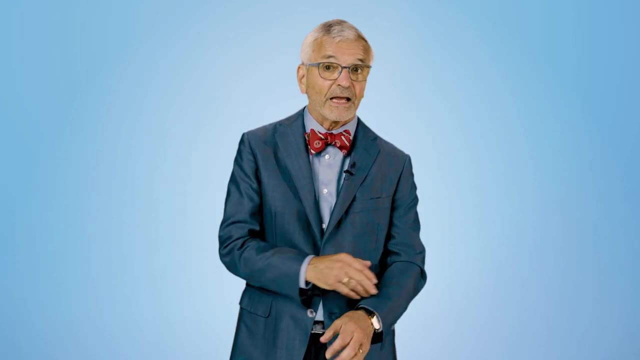 are very uncommon. In fact, patients with a history of non-anaphylactic egg allergies or contact dermatitis may have a history of non-anaphylactic egg allergies. A rash on the skin from neomycin can safely receive measles vaccination. 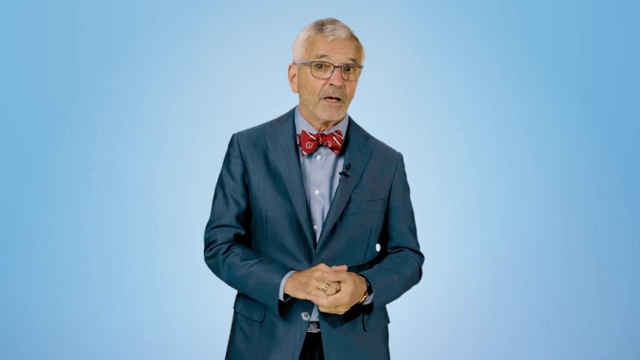 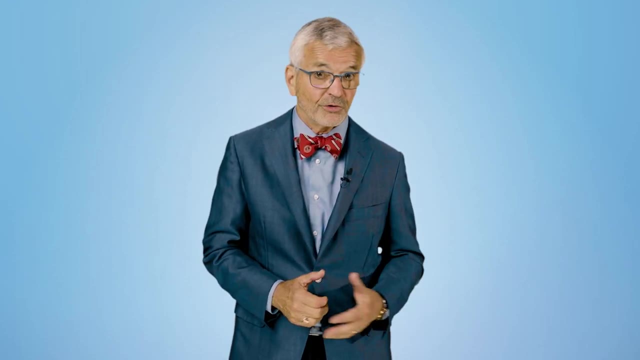 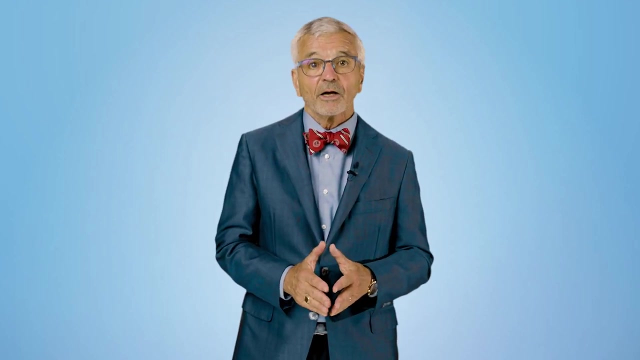 There are hypothesized associations or there have been hypothesized associations between measles vaccine and the development of inflammatory bowel diseases like Crohn's disease or autism. These associations have not been supported by many rigorously conducted and analyzed studies in the United States and around the world. 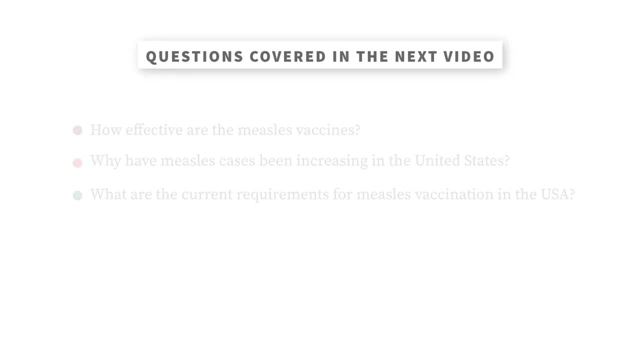 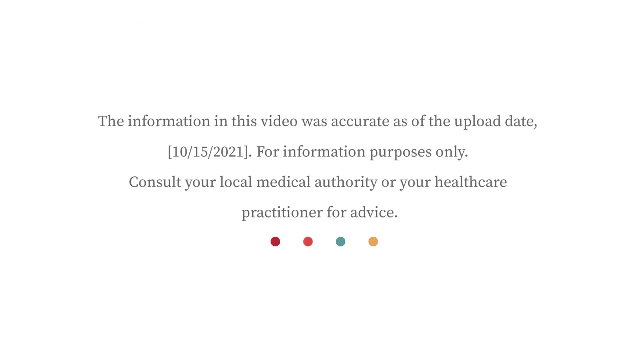 Questions covered in the next video: How effective are the measles vaccines? Why have measles cases been increasing recently in the United States And finally, what are the current requirements for measles vaccination in the United States?